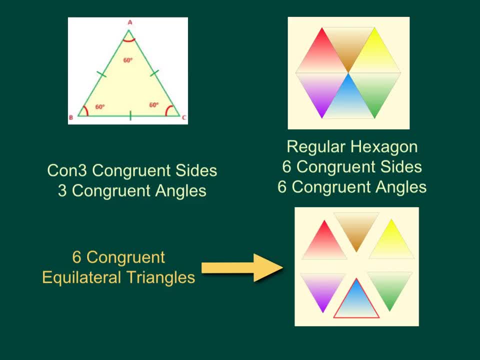 Okay, so just a quick introduction to the shapes. You probably want to draw these out, But the first shape up here in the upper left hand corner, this shape is what we call the equilateral triangle. Equilateral triangle, if you remember, has three equal sides, and three equal angles Should be saying concurrent. I guess That's an equilateral triangle. The other figure that we're going to talk about today is over here in the upper right hand corner. 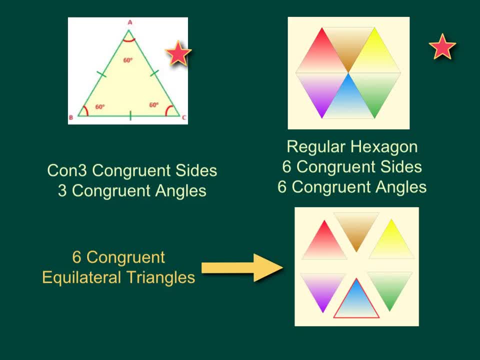 And that is our regular hexagon. Now, the regular hexagon has one, two, three, four, five, six congruent sides And the interior angles: one, two, three, four, five, six congruent interior angles as well. 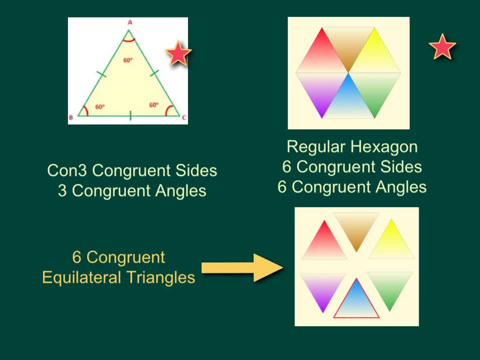 But the way we're going to talk about it, you know, if I can just focus your attention down here in the lower right hand corner, right there- We like for you to think of a regular hexagon as just being six Equilateral triangles. That way we'll only have one formula to memorize. 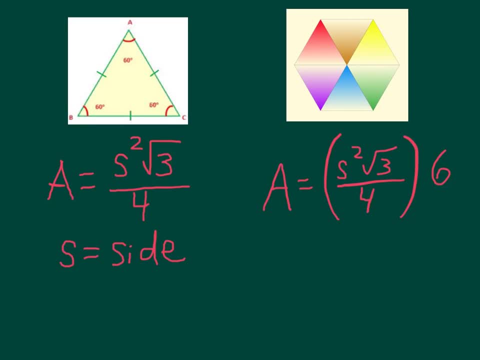 Well, speaking of those formulas, here they are. So the first shape is our equilateral triangle. The formula for the area of an equilateral triangle is: you take any side, we'll call it S square that side, multiply it by the square root of three and divide by four. 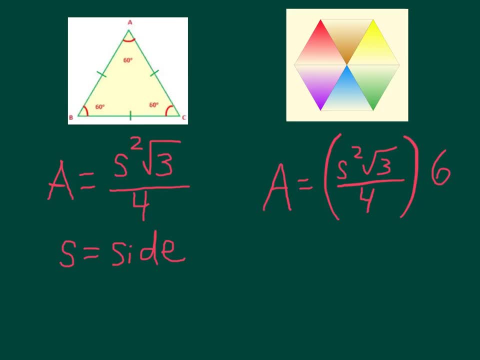 Now that probably sounds crazy. You're like: what about one half base times height? But just be patient, We're doing that on a coming slide. S- it's important to know that S stands for side, So I will highlight this. This is an S, not a five, And that is the side of the equilateral triangle. 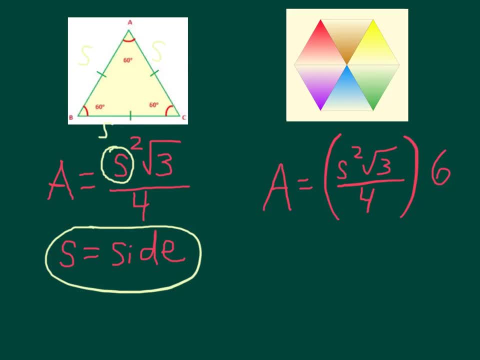 So S, S, S. Okay, that was a bad color choice, But S, S and S, And so those are sides of the equilateral triangle. Now when we come over here to the right hand side and try the regular hexagon, you know I can take anything. 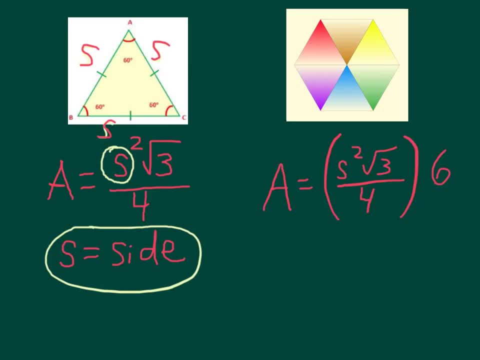 Basically, I want to find the area of maybe the square root of three. So I'm going to take this blue one. So, again, I'm using the same formula: the side squared root, three over four. And then what I'm going to do is, since there's a red, orange, yellow, green, blue, purple one, I'm going to just take that formula and multiply by six. 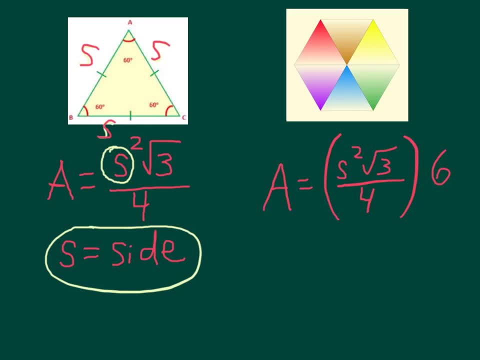 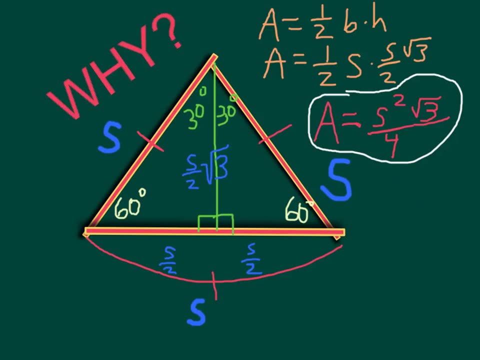 And that will be the formula you use for the area of a regular hexagon. So why is that Holy cow? Why is that? Well, you're probably looking at this slide and just freaking out, because there's all kinds of information. Okay, 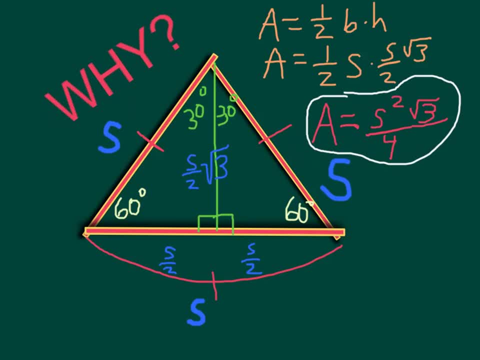 So what we did here was we drew an equilateral triangle. And so we have that. We have a side, a side and another side, Alright. And what we did was we dropped a perpendicular right through the middle. We dropped an altitude which, in an equilateral triangle, would split this in half. 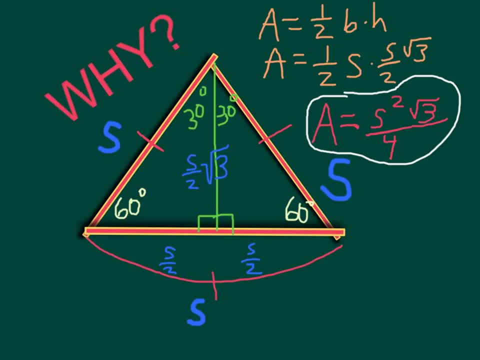 So side divided by two is side divided by two. Not only does it perpendicular bisect it, but it also bisects the angle up here to make them both. So that's what we're going to do with the side across from the thirty degrees. 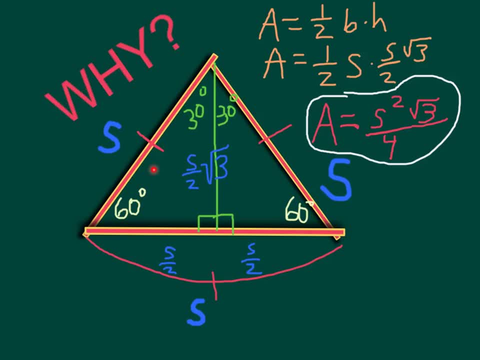 And so the rule we're kind of using here is, if the side across from the ninety is something, the side across from the thirty is half as much. So I should probably get those fancy arrows out. That was pretty cool. Um, the side across from. okay, maybe not the side across from the ninety. there you go. the side across from the ninety is s the side across from the. maybe I should make them smaller. 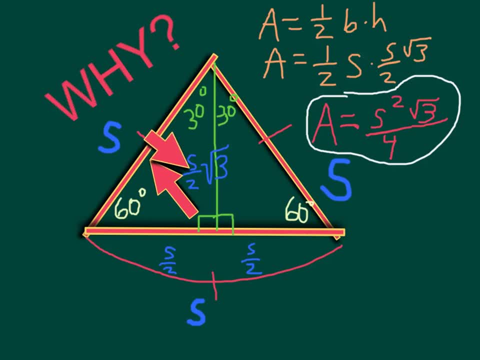 I don't know how to do that, but so the side across from the thirty is s over two. let's see if I can get them out of here. and then the side across from the sixty: um, as you look across there, um is going to be whatever. the side across from the thirty was times the square root of three. 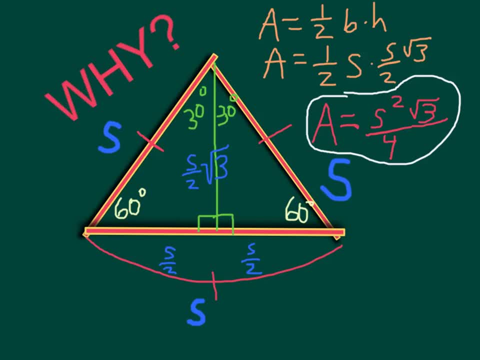 So this is a messy picture, um, but basically, when you simplify it? um, you're coming up with a triangle That has, you know, an altitude there that side, over two root three um a base of s? um, and we have other information as well. 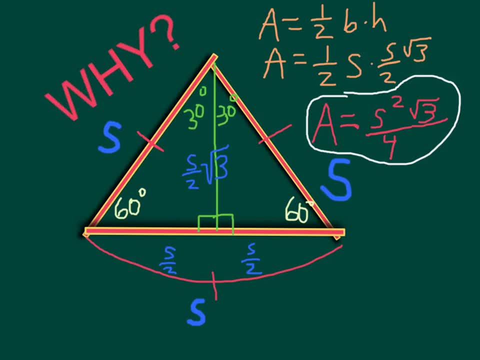 But I'm going to take you back just to the old area of a triangle. um, so that's this right here. If we take that and just look at the area as one half base times height, that's our old formula from the other day. 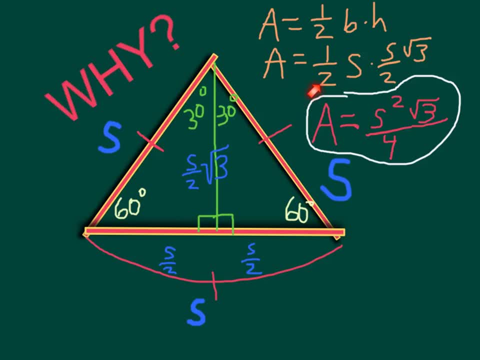 Uh, the area is one half, okay, the base, what's the base? The base is this thing. So, if that's the base, the base is just s okay. and what's the height? Well, this height we said was s over two root three, and so that's going to go here. 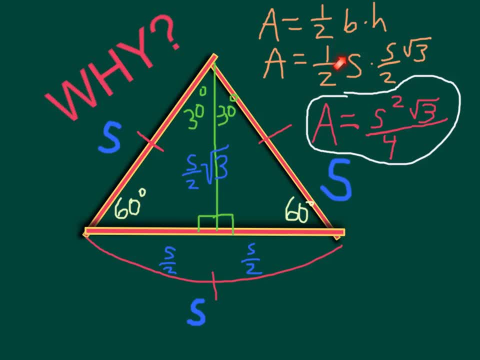 So the one half from our old formula. the base is the base of the triangle s and the height. we did a little bit of work to decide over um two root three, And so if you take s times s, you get s squared um. there's a couple twos in the denominator. 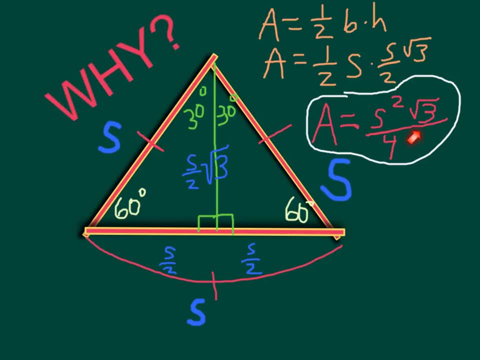 When you multiply them, you get four, And the root three is there as well. So it's side squared, root three over four. Now, um, I don't want to have to do all this work. I mean, the side itself just looks crazy. 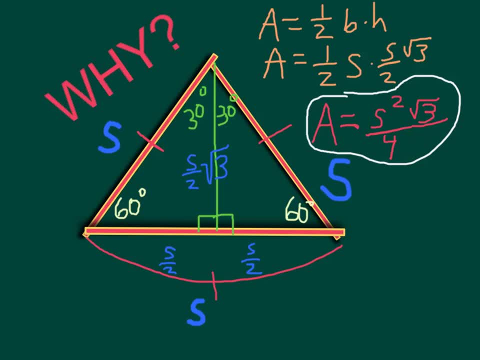 The slide itself looks crazy. So let's just go ahead and use this formula um and just kind of bypass this derivation from now on. So what I would want to do is just go ahead and use this formula right here. So how about a regular hexagon? 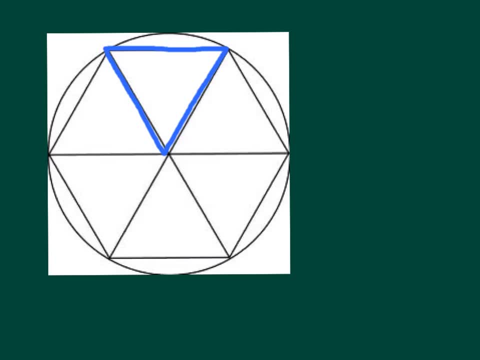 Why does that formula work? Well, um, the one we're using. um, we're going to use this formula. The formula we're using basically says that if you have an area of uh side squared root three over four, um, that we just derived on the last page. basically, you have one, two, three, four, five, six of them. 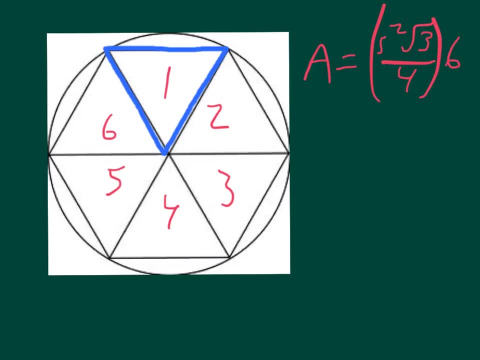 And so we're going to take that formula and multiply by six. Remember this thing right here: um, that is an s which stands for side. It is the side of the equilateral triangle. um, which also is the side of the regular hexagon as well. 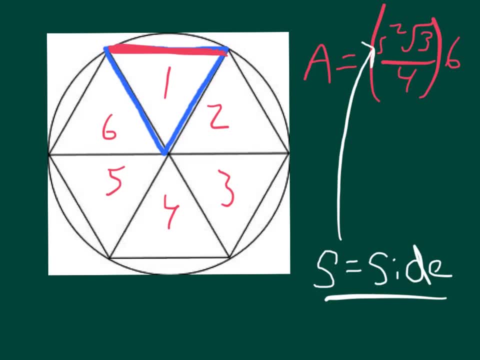 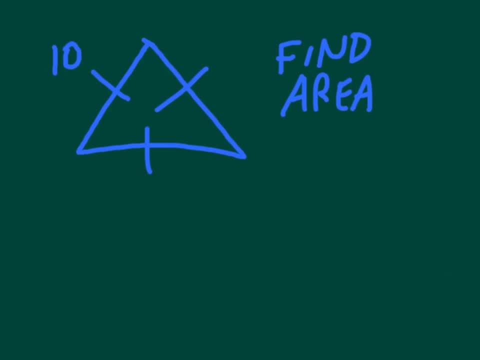 Alright, I had that inscribed in a circle just for fun, So we'd like to just do some straightforward problems. You might want to sketch this down. It's basically an equilateral triangle with side ten. I want you to find the area. 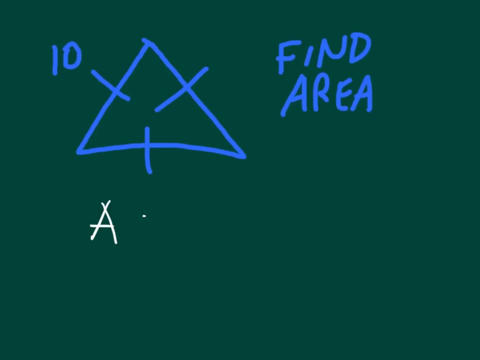 Well, okay, the area is equal to um side. Eh, I'm not following my own rules. Let me go back for a second. Okay, It's not going to. let me go back There, it is Alright. Um, the area in general is side squared root three over four. 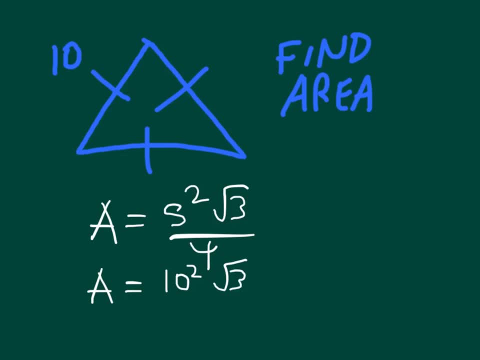 And then when I fill it in, it's ten squared root three over four, And so the area is equal to what is that? A hundred over four? twenty-five root three, And that's in square units. Alright, So that's a quick, straightforward problem. 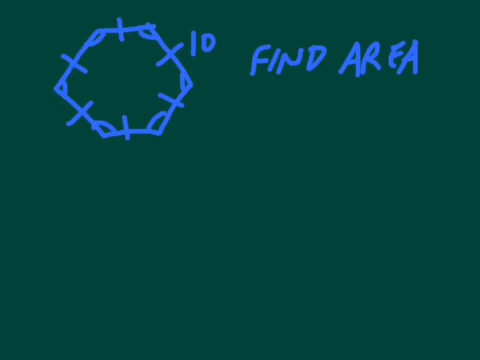 Our second problem here is a regular hexagon. Again, we just want to find the area. So what I'm basically going to do here in my answer, which will be in white pen again, um, I want to find the area of one little equilateral triangle. 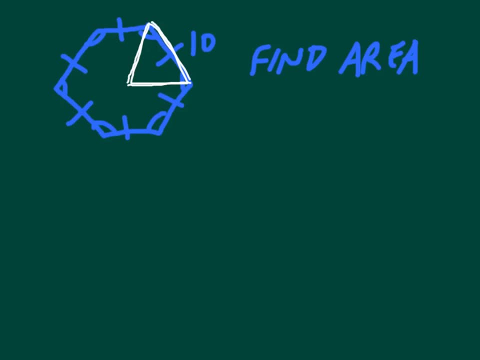 And then I know that I have six equal ones in there, So it is ten squared root three. Oh no, I didn't follow my own rules again. Let me erase that out there. Basically, what I'm going to be doing when I'm finding the area is I'm going to do seven. 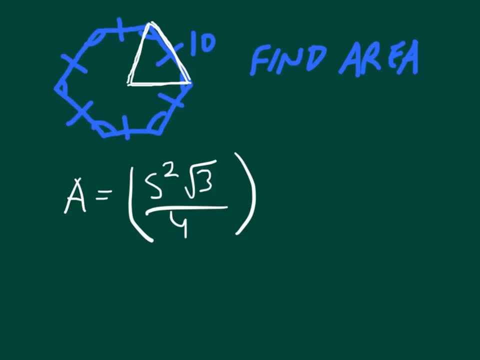 side squared root three over four, And then I have six of those when I'm done. So I feel like I did this a minute ago. I had like a ten in there. I got twenty-five root three, Um, and then now I have six of those. 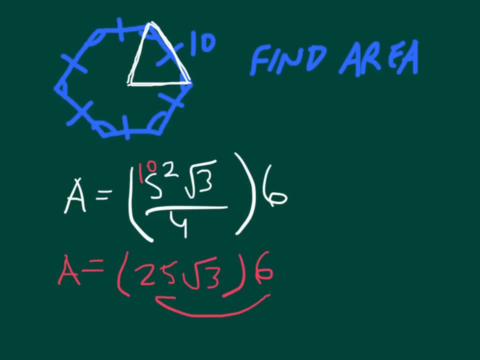 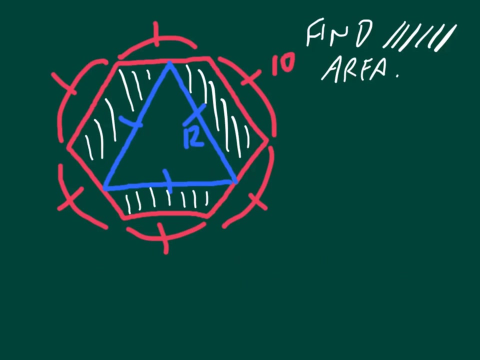 And the key here is only the number out in front gets multiplied by six, based on old rules. What is that? A hundred and fifty root three, And that's in square units as well, Alright, So here we have a more complicated problem. 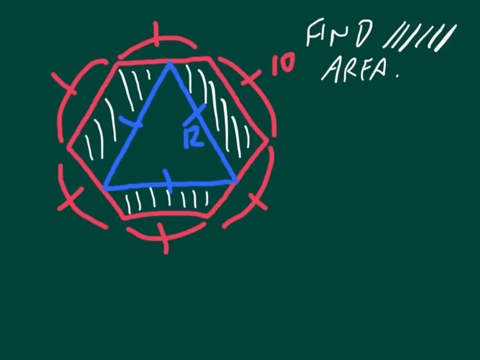 And I'm just going to write that: um, what was it? A hundred and fifty root three that we got for a regular hexagon with side ten, So I don't have to do that work again. Basically, we have this big um hexagon, um that we already know the area to. 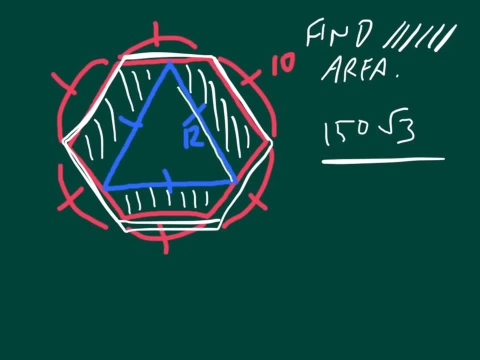 And what I did was something fancy in here. I just put an equilateral triangle inside, Alright, And so I want to know you know what's left over? You know what is this stuff Here and here and here. 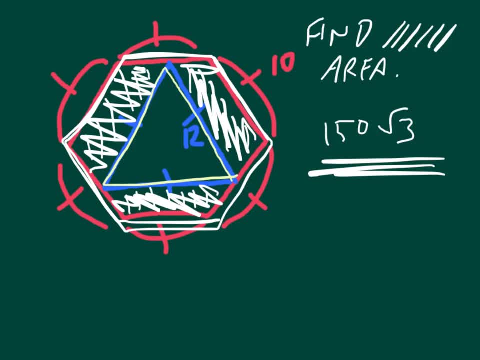 And so you want to say like, oh, it's a hundred and fifty root three, But uh-uh, that doesn't make sense because you want to subtract out, um, that area on the inside, So let's subtract out side. squared root three over four. 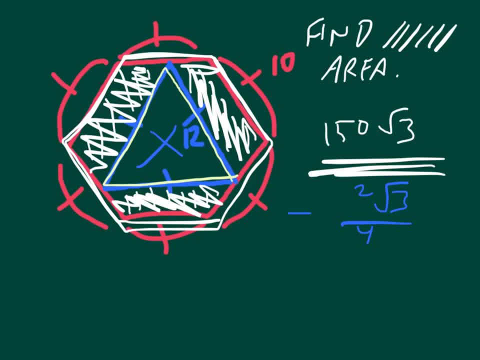 Um, that side is in our problem. twelve And so that's, you know, a hundred and forty-four. A hundred and forty-four root three over four. What is that? A hundred and forty-four, So seventy-two over two. 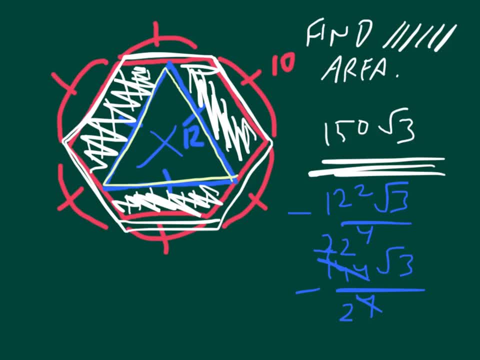 Maybe thirty-thirty-six, Maybe it's thirty-six root three. So, um, if I erase all of this, um, it ends up being thirty-six root three, Um, and so you have a hundred and fifty root three For all of this. 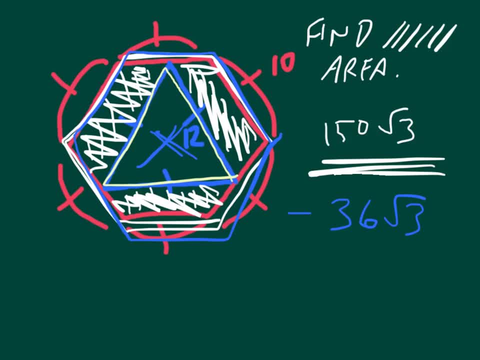 Okay, And then you take this middle part and subtract it out. So we got a hundred and fifty root three minus thirty-six. So what is that? Four gets us up to forty Fourteen, Maybe one-fourteen, I think it's a hundred and fourteen root three. 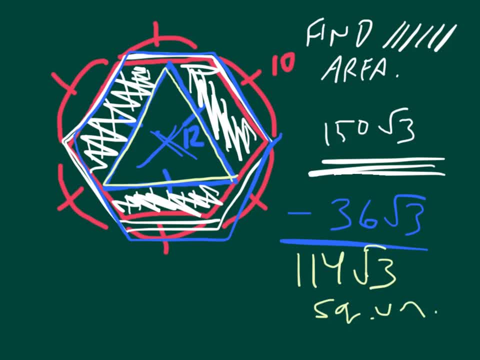 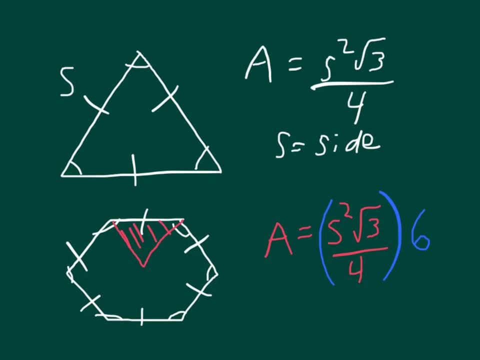 Um, and that would be in square units as well. Alright, And so that finishes that one off. Okay, Um, That came at you pretty fast and we're going to do some practice in a minute, but just a quick summary here. 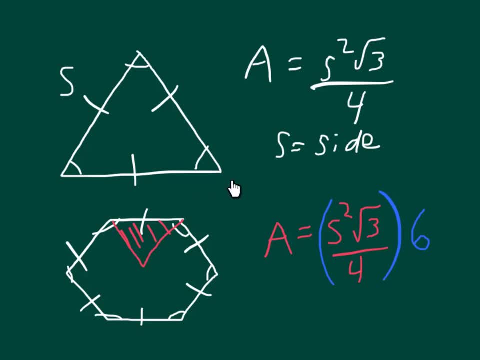 You know, in this first um problem, right here we have an equilateral triangle with three equal sides and three equal angles. Um the area of that is side. squared root three over four S stands for the side, So try to highlight it a few times, but this is not a five. 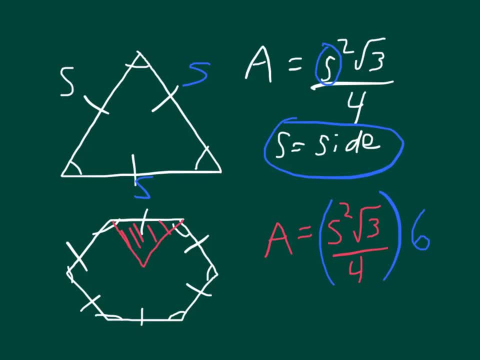 It is an S, It's for any side um of our equilateral triangle. Now, when you come down um here to Look at the regular hexagon, then, Um, what you want to do is just basically find one of those. 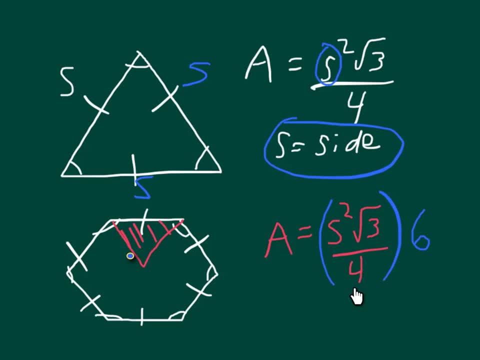 And then, once you find one of those, um, you plug it in here, Side squared root, three over four, That's a uh uh equilateral triangle. And you have one, two, three, four, five, six of them. 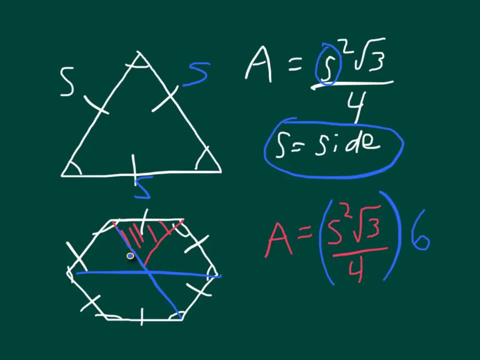 You just can't see them, but I can draw them in if you want me to. Um, and then you're actually going to be multiplying by six there to get your answer. And so those are our two formulas and hopefully they uh made some sense to you. 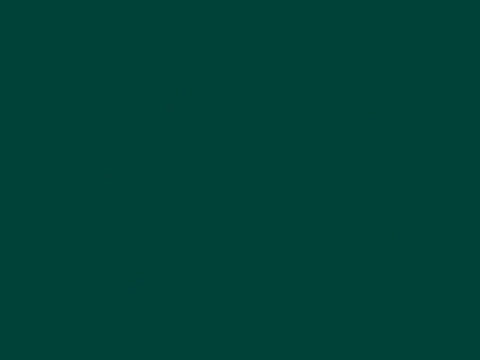 All right. Well, now we're going to have some time for questions. I don't know if you guys have any or not, Um, but we also have some questions for you guys. Enjoy the problems we have for you. Goodbye.